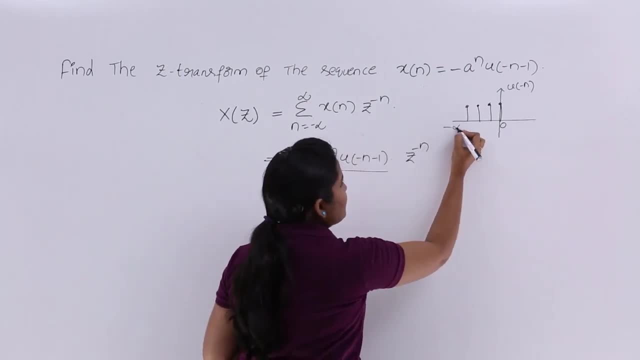 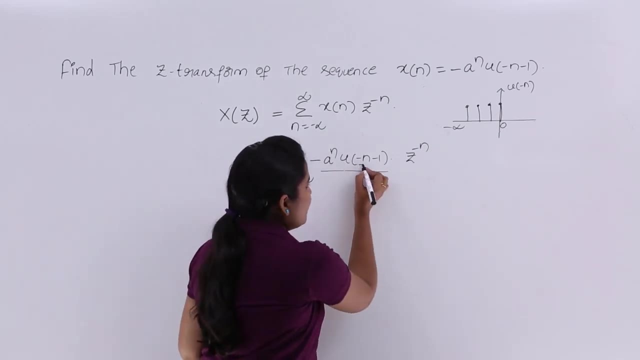 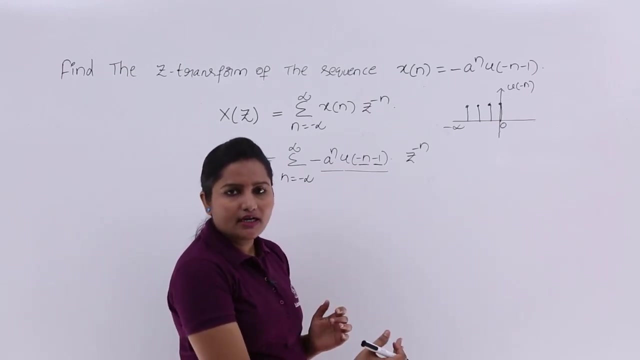 i plus little of z. Okay, infinity to 0.. This is general left sided unit step. For this left sided unit step we are having shift of minus 1.. Shift of minus 1 means that is a positive shift, or negative shift means that is. 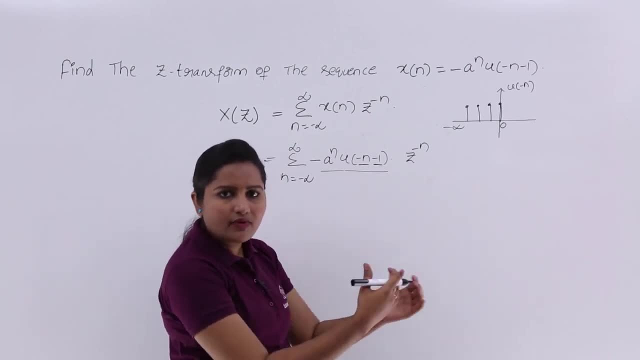 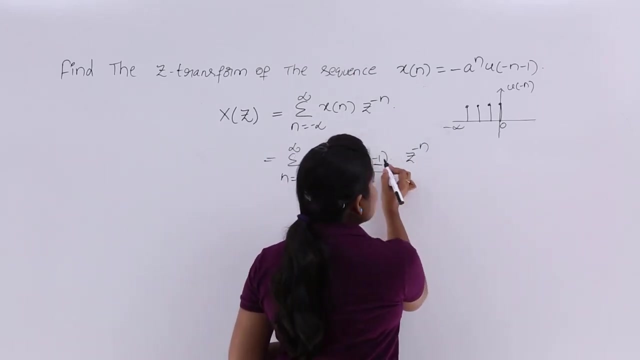 positive shift. When you are having minus value, that is a positive shift. When we are having negative value, that is a left shift. So here we are having negative value, So we are having right shift. So here that right shift is 1. position u of minus n, minus 1 is right shifted. 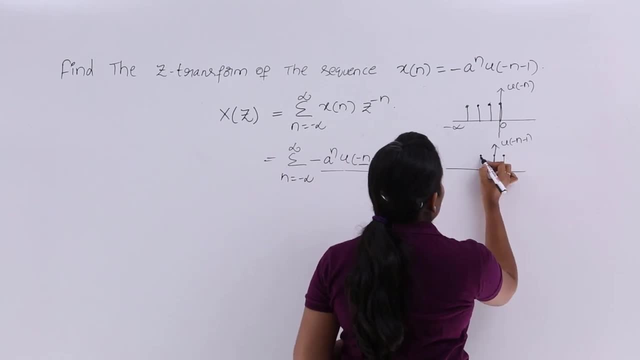 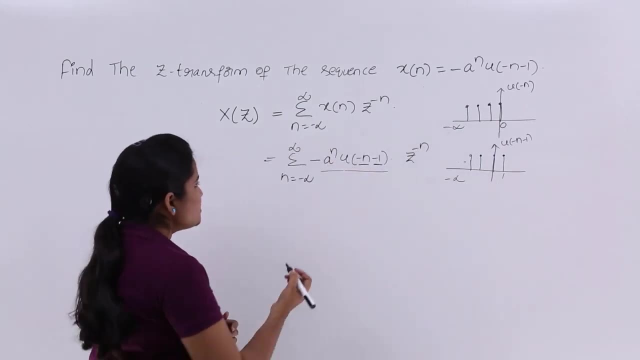 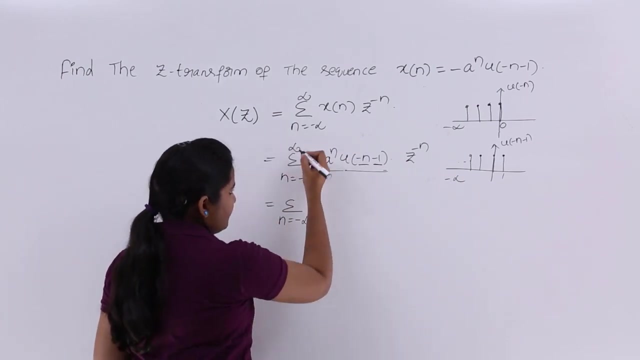 to 1 position means so here this will be your resultant signal. So minus infinity to 0 will change to minus infinity to 1.. So this unit step function will changes this summation from minus infinity to infinity to minus infinity to 1.. In this region the 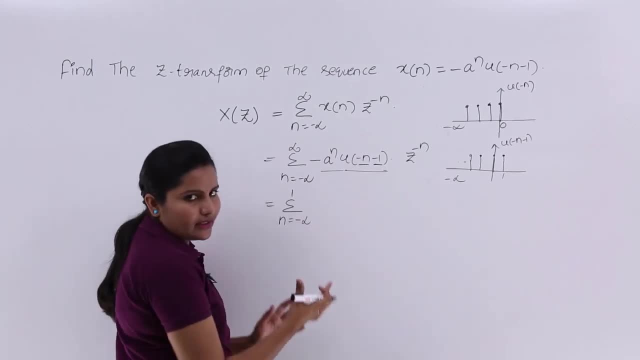 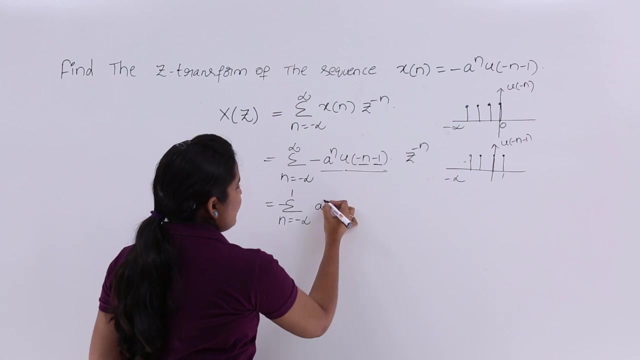 unit step function value is equivalent to 1. no need to write in the next step, because so 1 into this thing will become 1. that a power n into z power minus n, only So that minus. I am writing outside a power n into z power minus n. I am writing like this, a inverse. 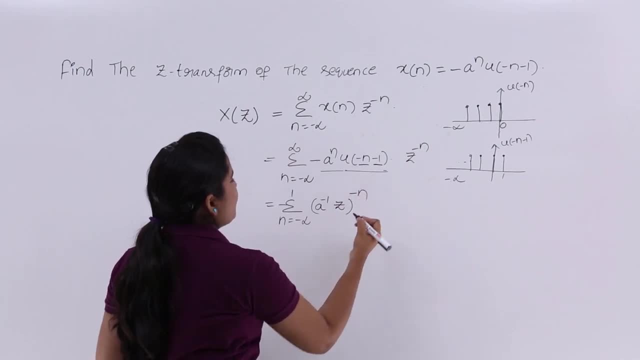 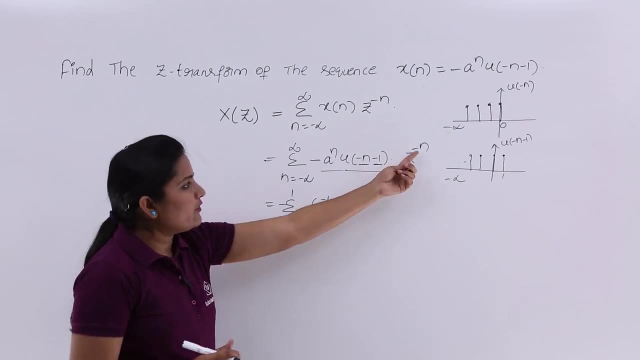 z whole n. So a inverse: z whole power minus n. I am writing like this: I take in common of this: a, z whole power, n. for z I am having negative n power and for a I am having positive n power. So that is why I written a inverse z to write the power equivalent to minus n. So a inverse. 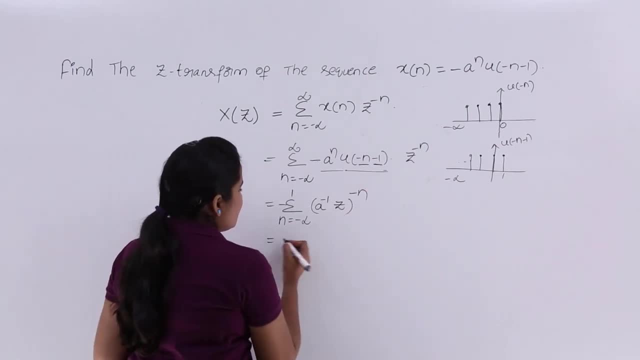 z, whole power minus n. I written like this: So now I can change this summation. So if I want to change this, I can change this. So if I want to change this, I can change this summation like this: n equal to 1, 1 to infinity. if I want to change this or reverse. 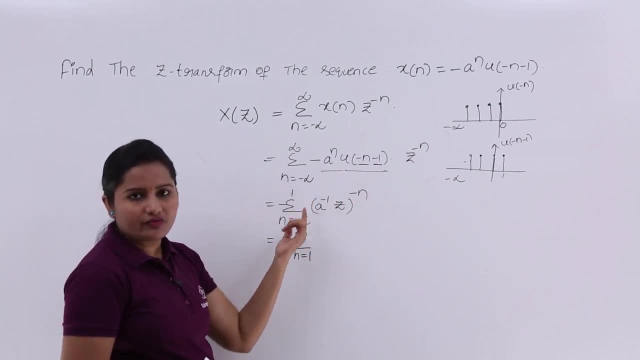 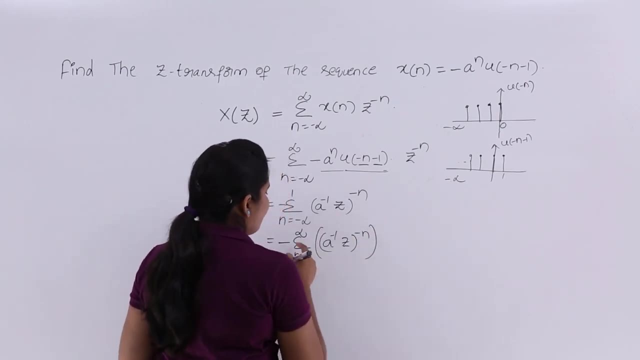 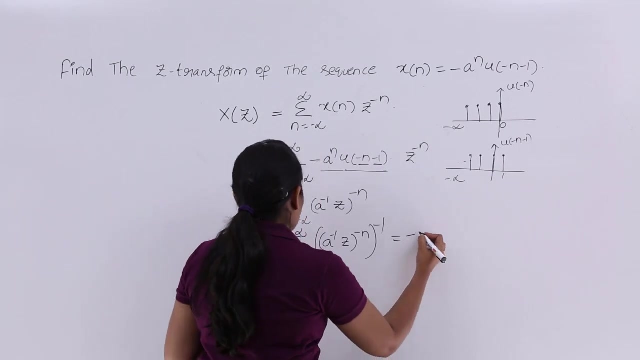 this summation. So I need to consider inverse of this. that means a inverse. z whole power minus n is already there. if I want to write like this in reverse, I need to consider like this: So that is equivalent to minus summation, n is equivalent to 1, to infinity. a inverse. 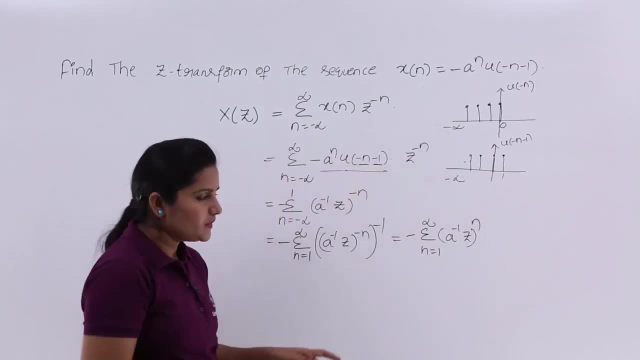 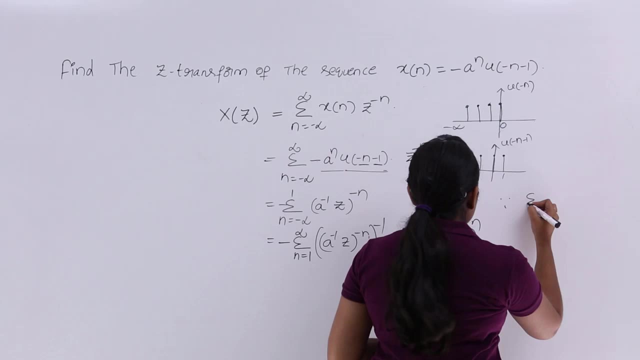 z whole power n minus n into minus 1, you will get n. but we are having equation for summation n equal to 0, to infinity. So a power n. we are having equation as 1 by 1 minus a. this is the fundamental equation we are already having. 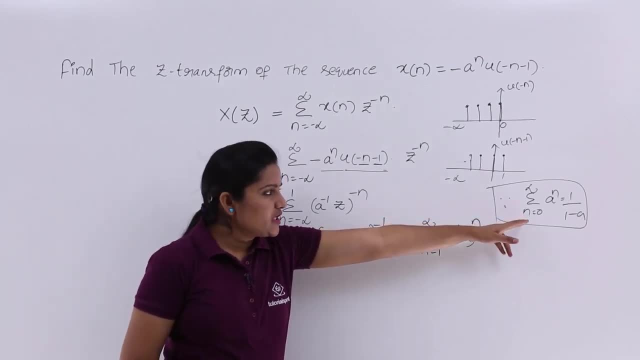 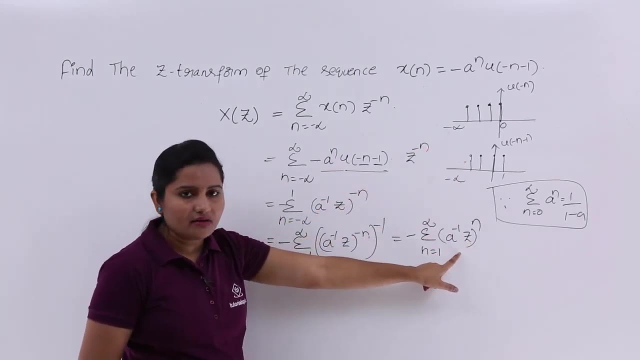 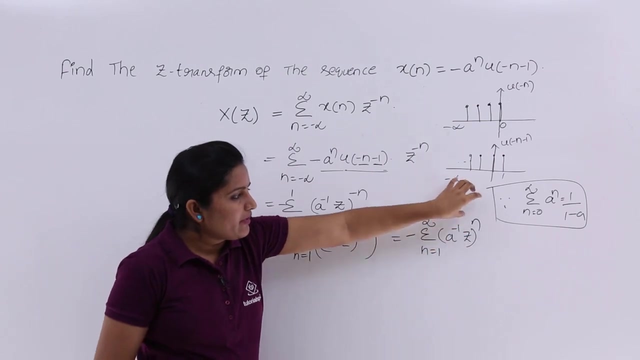 We know this: since summation n equal to 0 to infinity, a power, n is equal into 1 by 1 minus a. here i need to have this summation limits from n equal to 0 to infinity. here i am having a power. 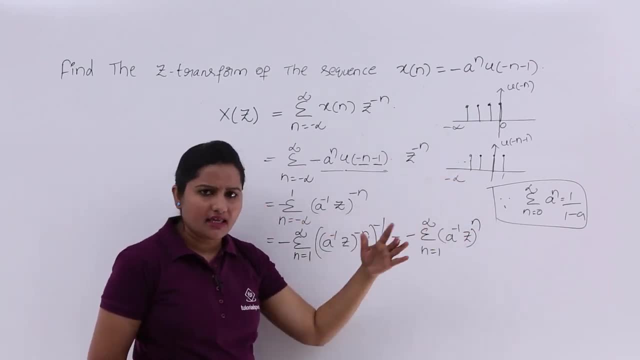 n form, this total thing. you just consider like a and that is in a power n form or x power n. for example in the equation, if you are having x power n- 1 by 1 minus x t power n, 1 by 1 minus t n power, 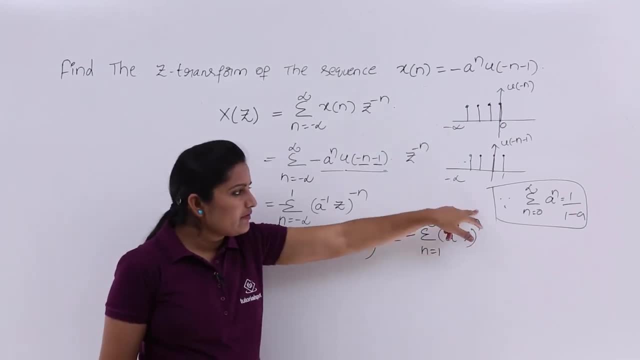 n 1 by 1 minus n, like that. so here i am having this form, but in summation limits i am having problem. so here you can see, i am including that summation n equal into 0 to infinity, a inverse z, whole power n. i included n equal to 0 term, even though that is not having actually 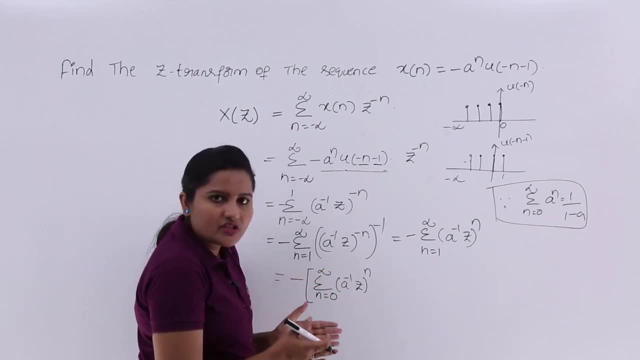 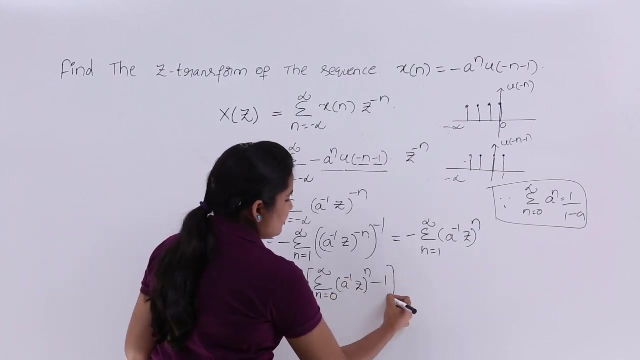 whenever i included any term which is not we are having in actual, we need to subtract that. so i am subtracting that n equal into 0 term here, so n equal to 0 term. if you substituted in this, so you are going to get minus 1. that means a inverse z whole power. 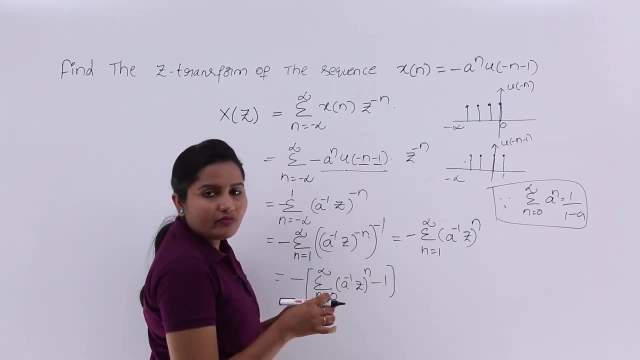 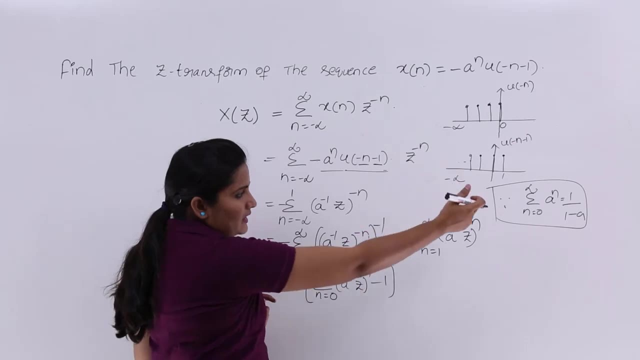 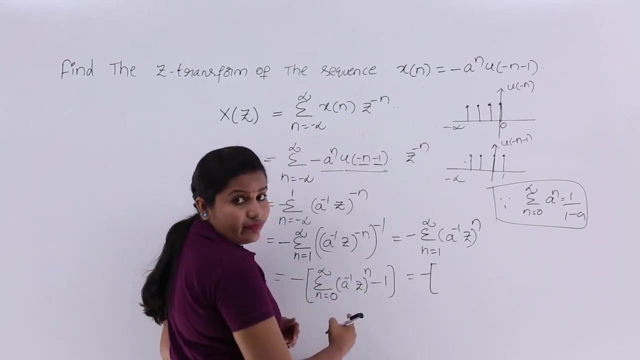 0, anything, power 0 is equivalent to 1, so the term equivalent to n, equal to 0, is equivalent to 1. so like this, you can write this one to apply that formula, so this is equivalent to minus. so here now, this will this, this we are having in this type of formula. 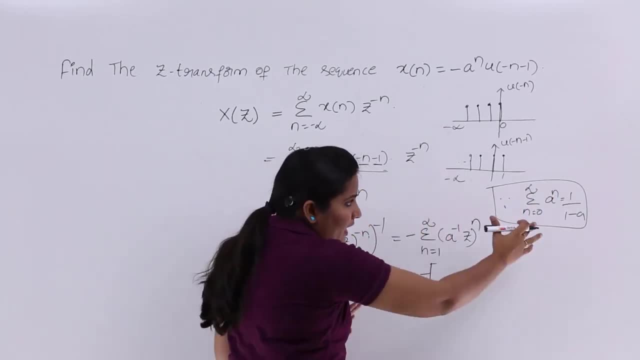 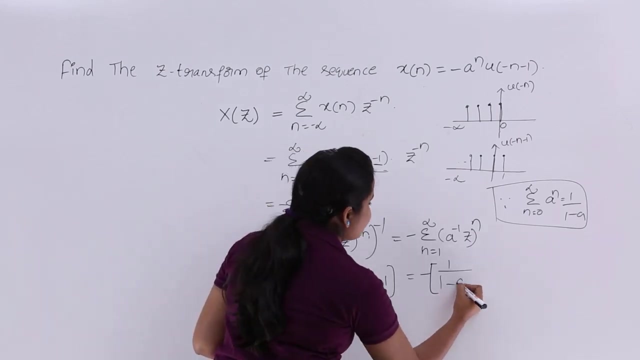 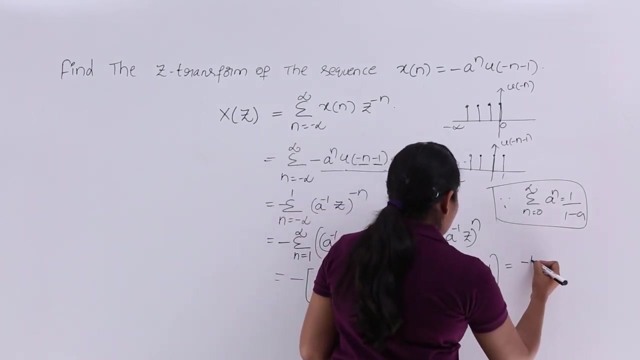 so we can apply this summation: n is equivalent to 0 to infinity, a power n formula here. so now that is equivalent to 1 by 1 minus a means. in the, in the place of a we are having a inverse z, a inverse z and minus 1. you are having now this is equivalent to minus 1. 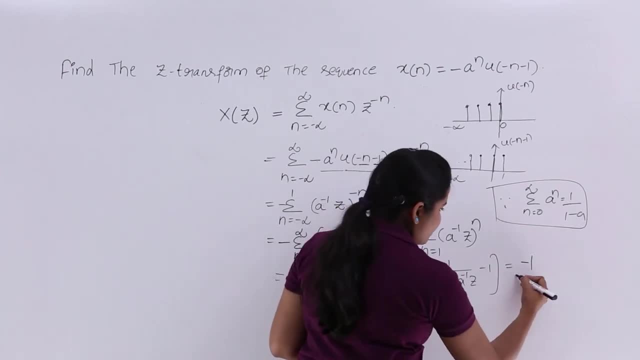 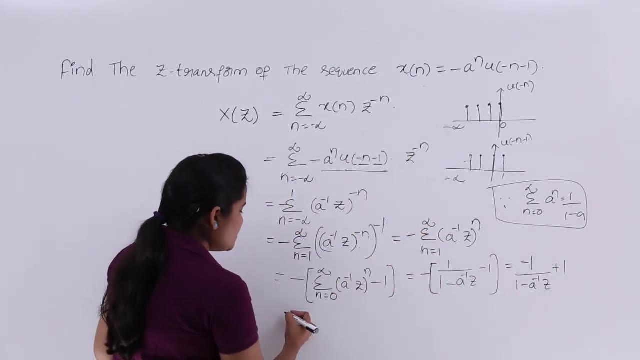 so I am adding this: minus 2 inside 1, minus 1 minus a inverse z plus 1.. Now cross multiply so minus 1 plus 1 minus a inverse z by 1 minus a inverse z. So now this is equivalent to minus 1 plus 1, gets cancelled and here z minus. 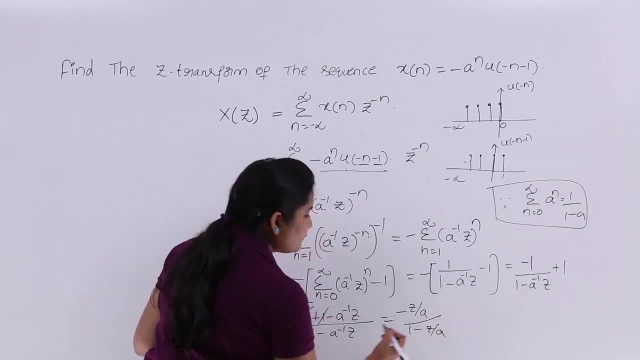 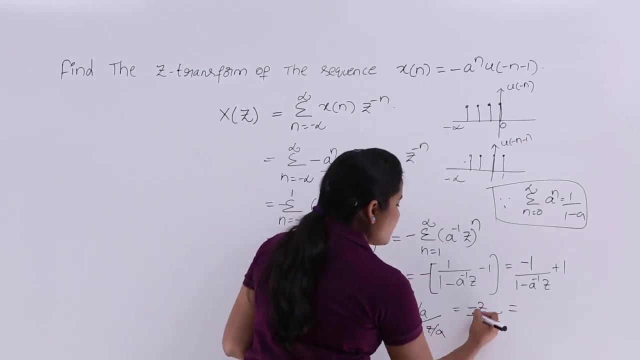 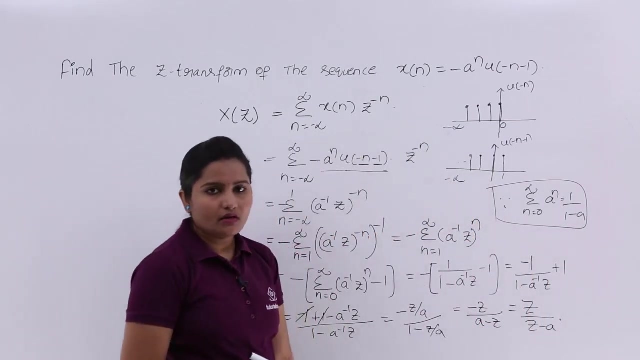 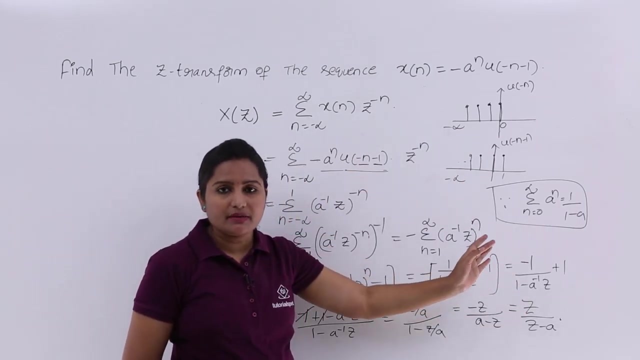 z by a by 1 minus z by a. So this is equivalent to minus z by a minus z. this minus. if you send to denominator, that is equivalent to z by z minus a, For example, if you are not having that minus, you will get minus here. that means z by a. 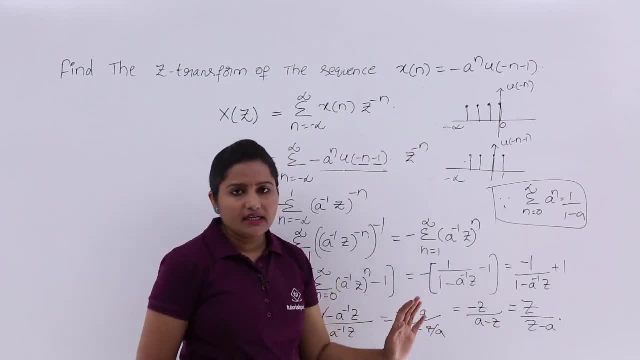 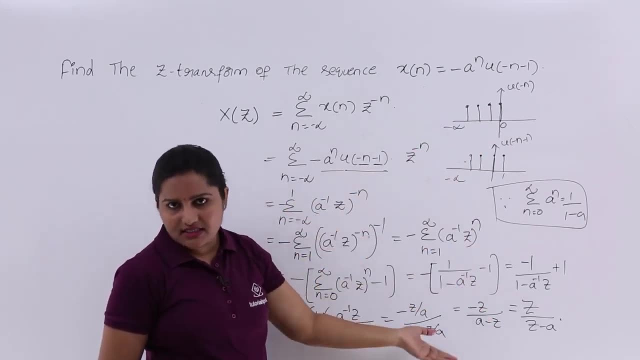 minus z only you are going to get. So generally they will give it minus like this: minus a power n? u of minus n minus 1 form they will give: If minus is not given z by a minus, z will be your transform. So now, this is the fundamental signal you are. 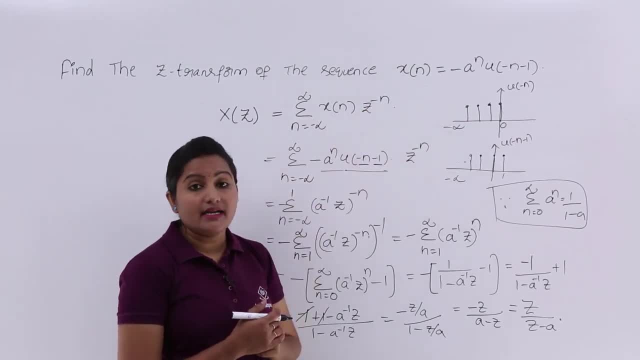 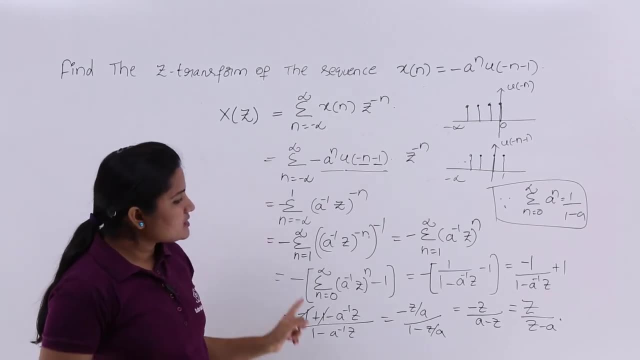 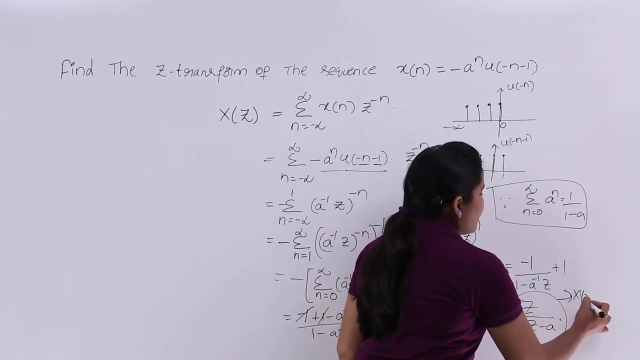 having x of n is equivalent to minus a power n? u of minus n minus 1. for that the z transform you got as z by z minus a. So all this is x of z. Finally you got x of z is equivalent to: this is x of z, for the signal minus a power n? u of minus n minus 1 will be z by. 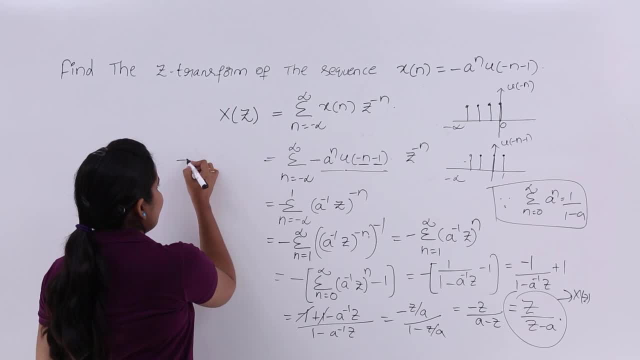 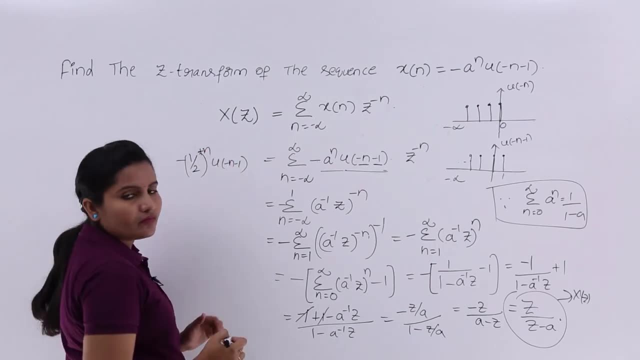 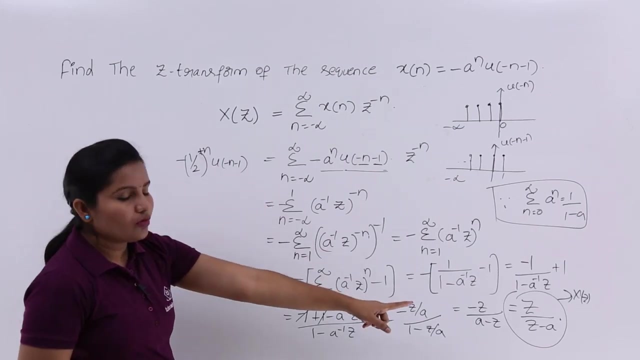 z minus a. For example, in any exam they are asking like this: 1 by 2 whole power n? u of minus n minus 1.. When you saw positive power, when you saw positive power on the value and you are having negative unit step function, then you can go for this transform. So I 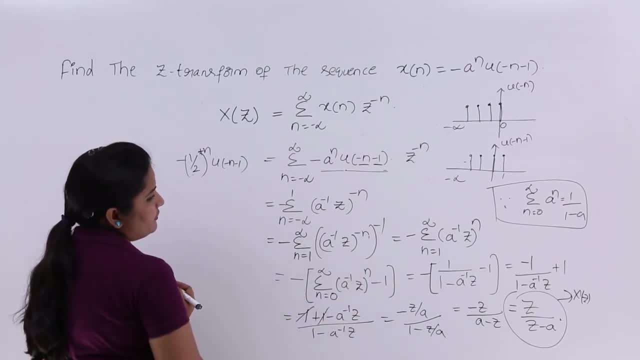 am substituting 1 by 2: whole power n? u of minus a power n? u of minus a power n? minus a Asian, so z by z minus n. 2 x a? u of since 1, the second số z is 1 by 2 in place of a.